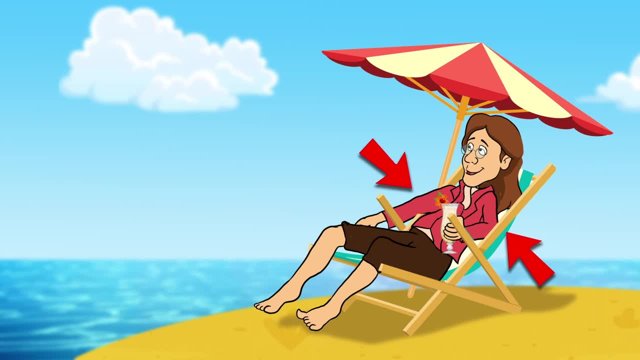 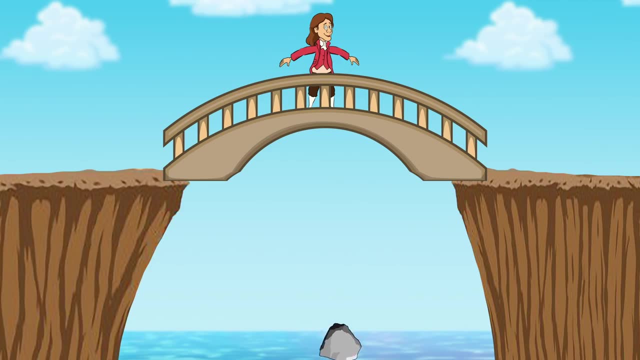 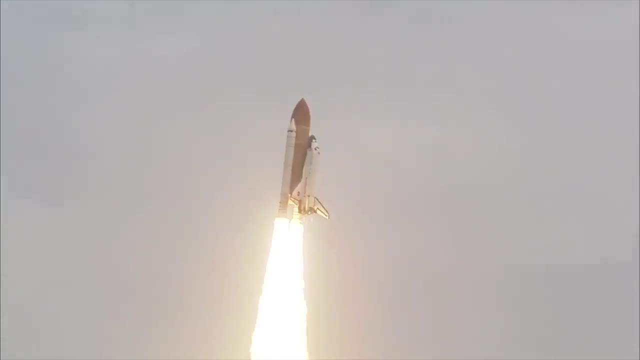 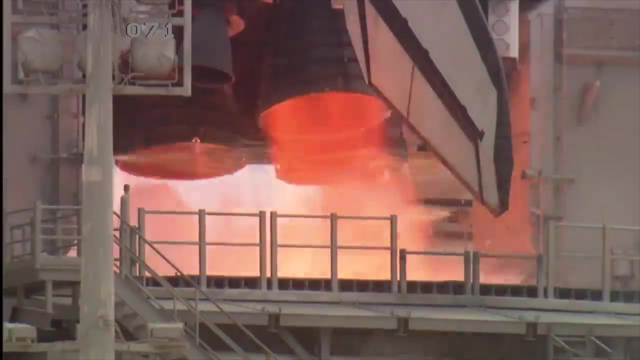 no matter how little the objects are moving, And sometimes you can really see an action and a reaction. In Florida, at the Kennedy Space Center, scientists use rockets to launch space shuttles into orbit. When the rockets fire, the exhaust from the rocket moves downward. 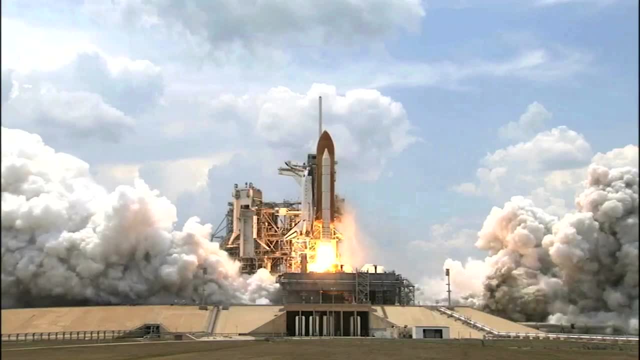 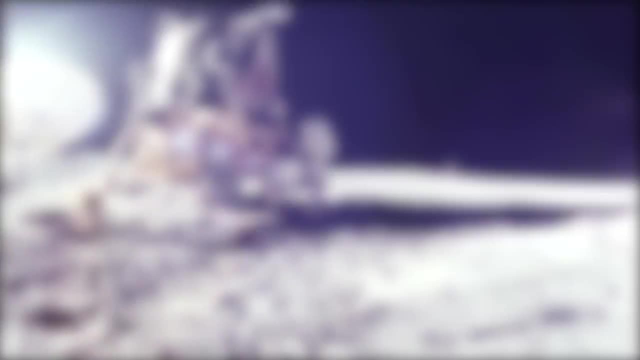 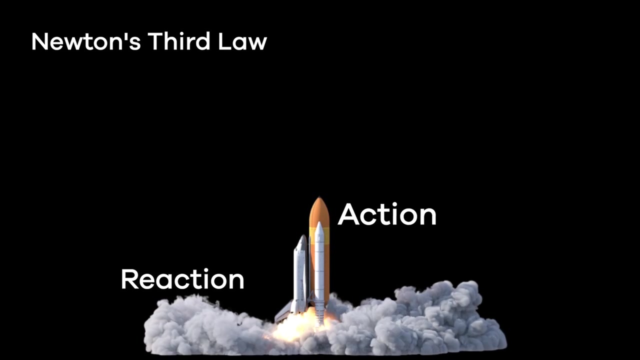 while the rocket moves upward. Without this law of motion, the space shuttle would never have lifted off the ground And we would never have landed on the moon. The force of action and reaction working together caused the shuttle to launch. You can't have one without the other. 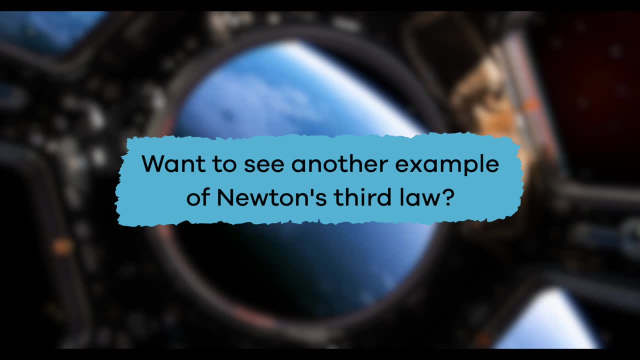 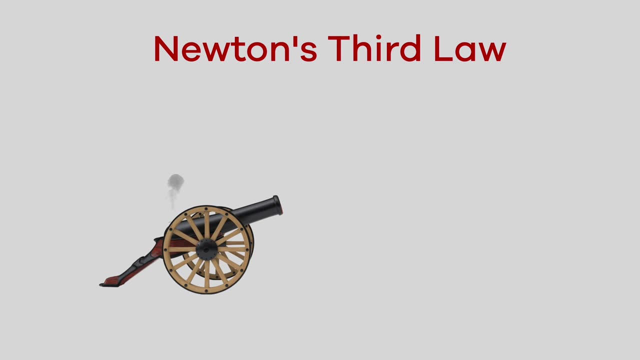 Want to see another example of this. Want to see another example of Newton's third law. What do you notice This time? let's slow things down and see if we can identify the action and reaction force. Did you notice that the cannon moved backward when the cannonball shot forward? 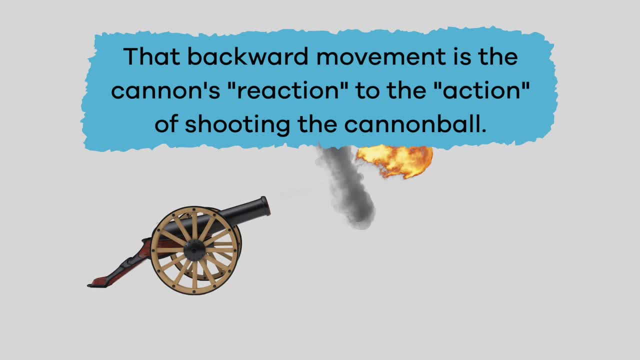 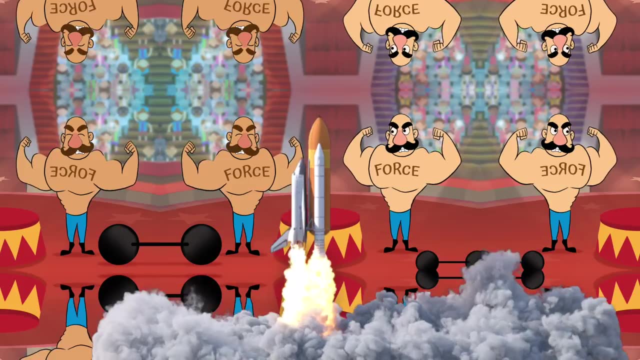 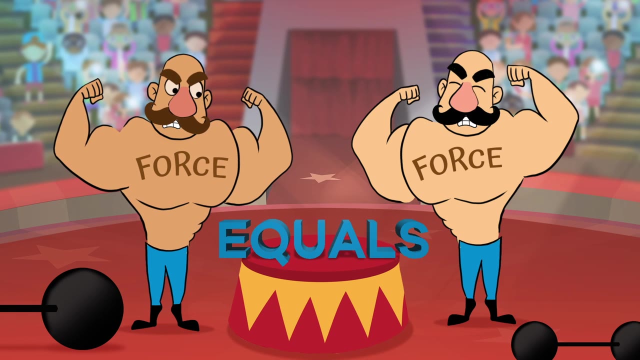 That backward movement is the cannon's reaction to the action of shooting the cannonball. Just like with the space shuttle, Newton also noticed that the cannon's reaction to the action of shooting the cannonball was the same as with the space shuttle. Did you notice that the amount of force on the first object always equaled the amount of force on the second object? 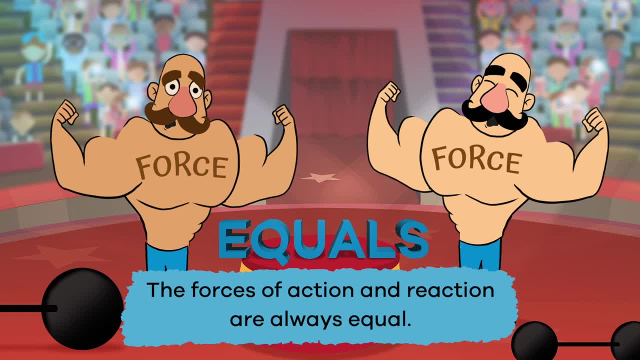 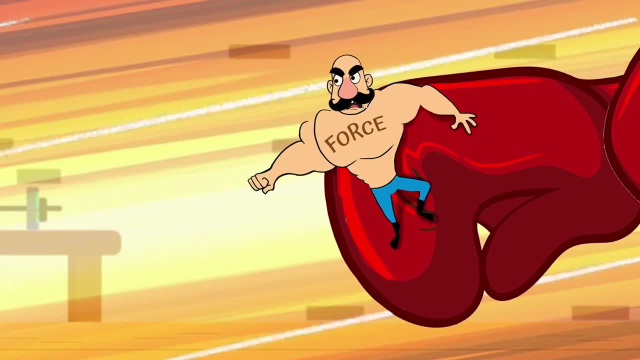 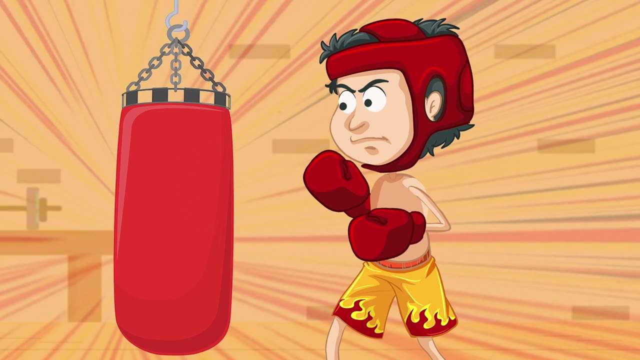 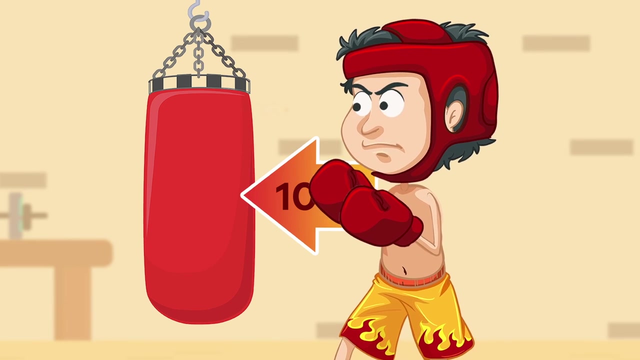 In other words, the forces of action and reaction are always equal. That means if a boxer punches a punching bag with 50 pounds of force, that punching bag will also hit the boxer's fist with 50 pounds of force. Ouch, If the boxer only gives 10 pounds of force with his fist, his fist gets 10 pounds of. 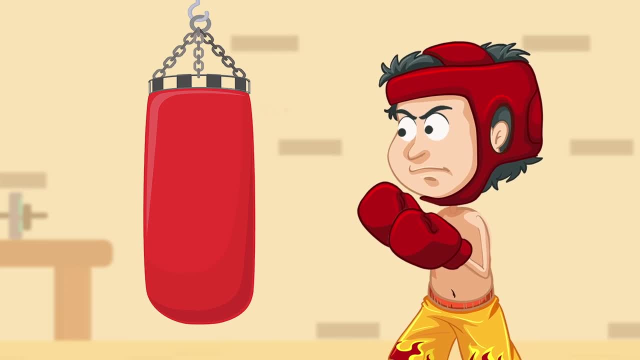 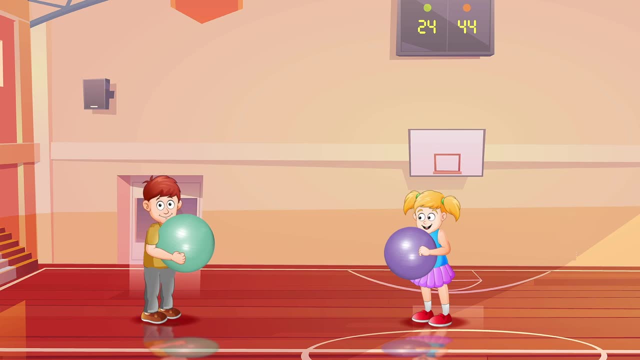 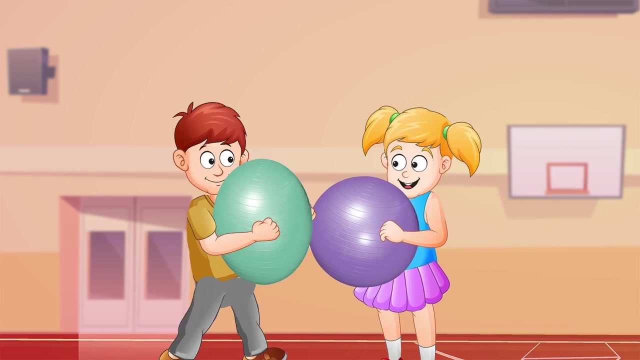 force in return, And if he gives 5 pounds of force, he'll get 5 pounds of force back. So if the forces of action and reaction are always equal, how do you think this is going to end? Ugh, maybe don't try that one at home. 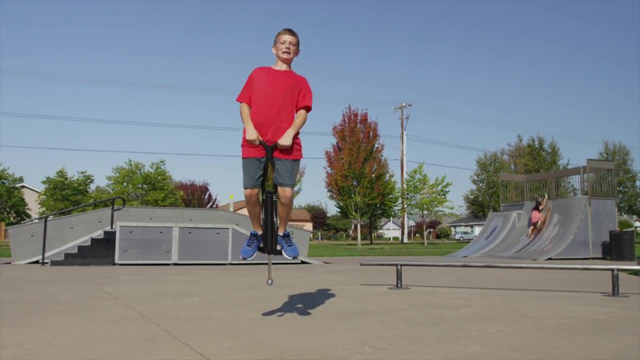 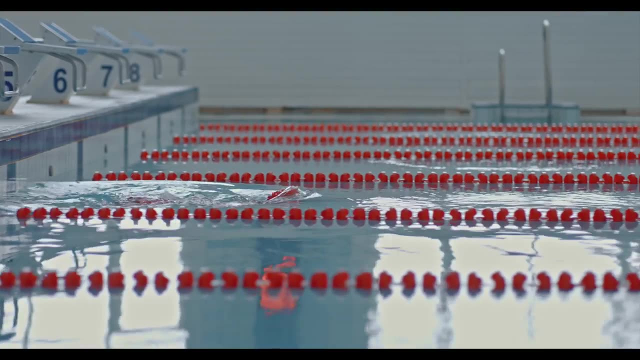 Now that you know about actions and reactions, let's move on to the next lesson. Let's move on to the next lesson. Think about the many reactions we cause every day. Let's talk about one last thing. Have you ever tried to move a heavy piece of furniture like a couch?